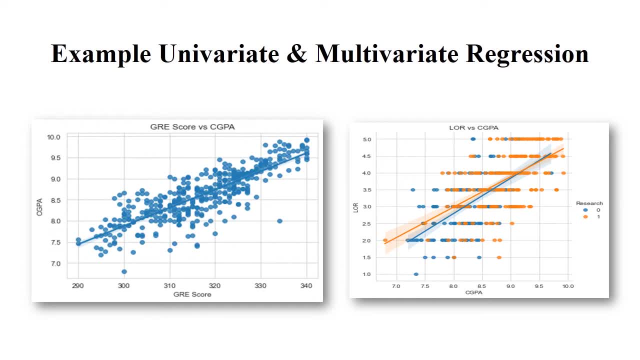 here, in this example, the first diagram, just focus on the first diagram. on x axis there is GRE score. on y axis there are CGPA, Right. So there are only two variables are there? CGPA is depend on GRE score, So CGPA is dependent variable. GRE score is independent variable. and this graph, this regression, show the relationship between that. So this concept is called as univariate regression. Now see in another diagram. 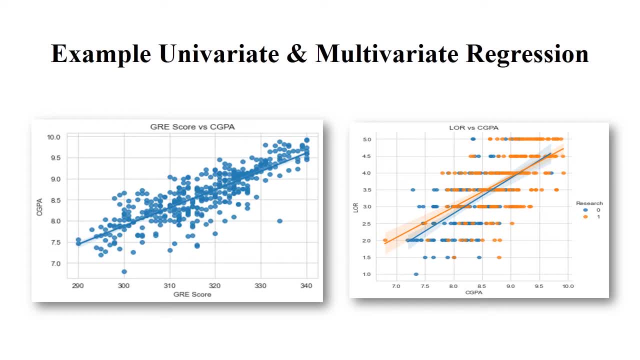 So on x axis, CGPA, y axis, LOR. Okay, So that is later of record, that is LOR. Okay, So LOR is depend on CGPA. But now see here, there is again another independent variable is there, that is research. So research means blue means zero means the particular person not interested in research, Orange means one, One means interested in research, Right? So according the relationship between LOR and CGPA, they again show the research interest. 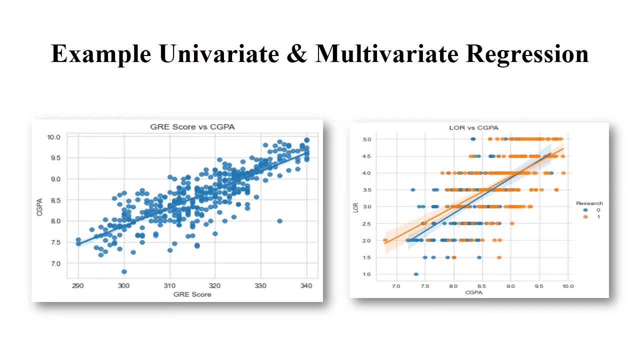 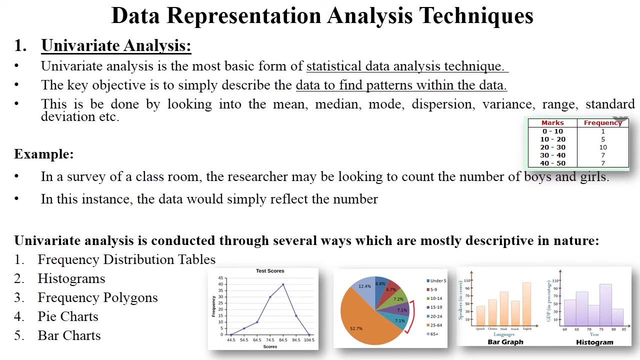 So blue color dot is not interested in green color dot is interested, See here. So means there will be more. There are more than one independent variable, is there Right? And LOR is dependent variable, CGPA and research is independent variable, So this concept is called as multivariate regression. Next Now there are some data representation analysis technique. So first one is univariate analysis. So univariate analysis technique generally uses. 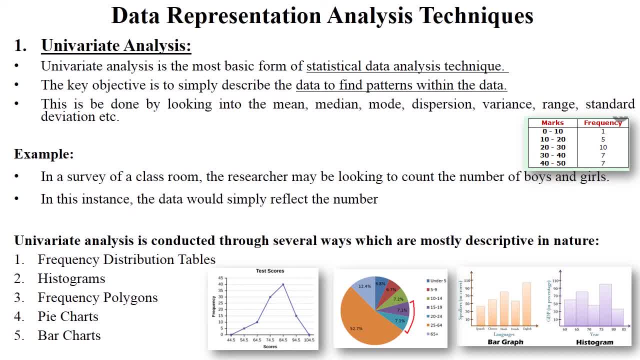 some statistical data analysis technique. Right, They show all the data and they represent the data in statistical format. So they describe the data in particular pattern and particular format. And this is done by to calculate a mean median mode than variance range, standard deviation. So this, all things are called as univariate analysis format. So see here these are some graphical format. First is frequency distribution table means zero to 10 marks. frequency distribution table. 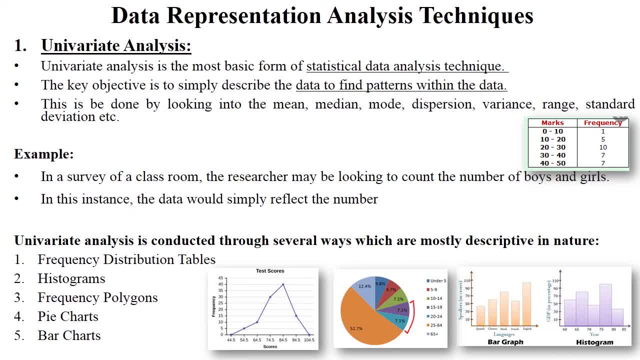 Next is one one student: zero to 10 marks. 10 to 20 means five students get 10 to 20 marks. So this is a univariate analysis. OK. Frequency distribution table is example of univariate analysis. Next example is a histogram. See here in the histogram there there are bar graph and histogram. This is example of univariate analysis. Next one: frequency polygons, pie charts- OK, And bar charts. So these are the representation of univariate analysis. 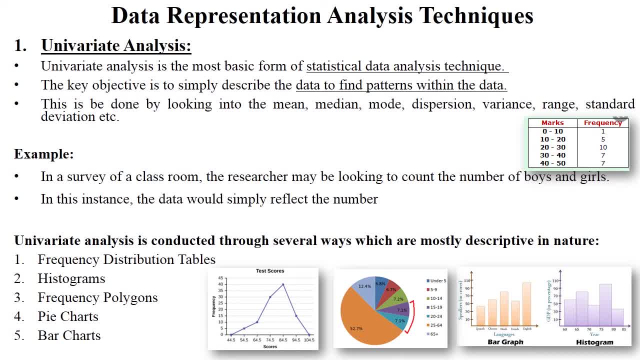 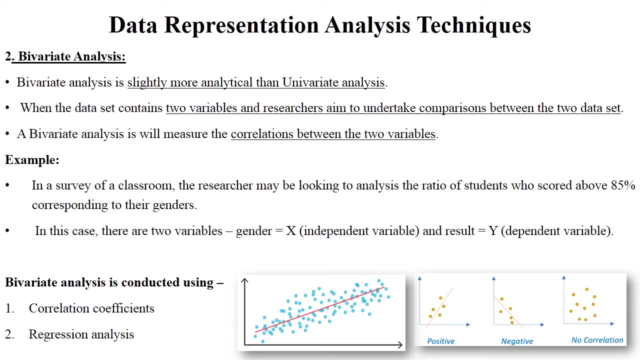 And again one example: Suppose there is a one classroom, OK, And the researchers may be looking to count the number of boys and girls. So this number of boys and girls reflected in particular number Right. So this is a univariate analysis, and univariate analysis represented in the format of frequency distribution table, histogram, polygons, pie chart and bar chart. Now the next representation analysis technique is bivariate analysis. So bivariate analysis is more analytical than univariate analysis. 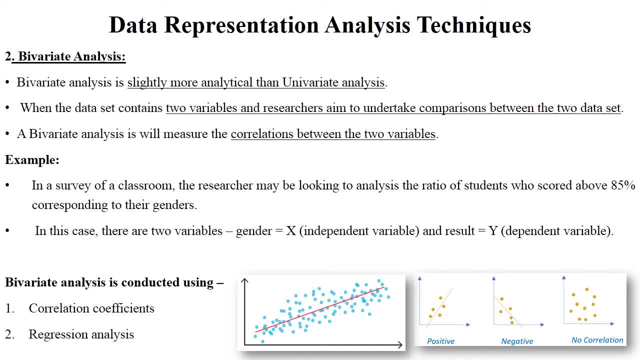 Bivariate analysis technically used. OK, See here in this below diagrams. These are the some regression diagrams are there. First diagram shows the regression technique. The second diagram show positive regression, negative regression Right, No correlations are there. So for regression representation purpose bivariate analysis technique is used. So bivariate analysis technique. there are independent and dependent variables and the relationship between that. So these are the bivariate analysis. 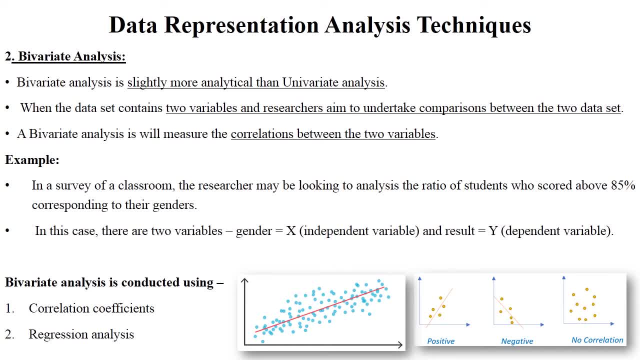 That is a first diagram represent as correlation coefficient and second diagram is known as regression analysis. So this is an example of bivariate analysis. For example in survey or classroom. Suppose the particular research. look a student who scored above 85 percent Right. So above 85 percent is particular condition. So there are two variables: gender and result. So X is independent variable and Y is dependent variable. So these are the examples of bivariate analysis.